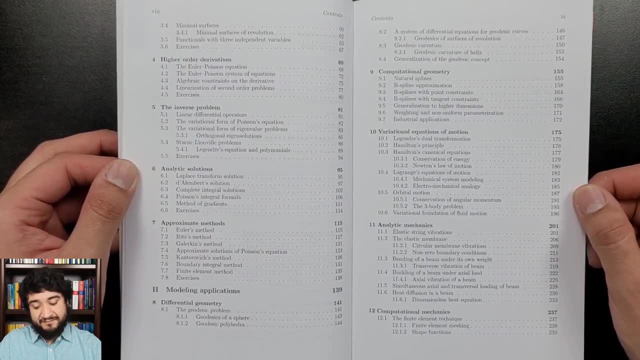 point. It emits a lot of technical detail, Something that I dislike about the book. sometimes I think it's a little bit too much. but it's a little bit too much. Sometimes I think it's a little bit too much. Sometimes I think it's a little bit too much. 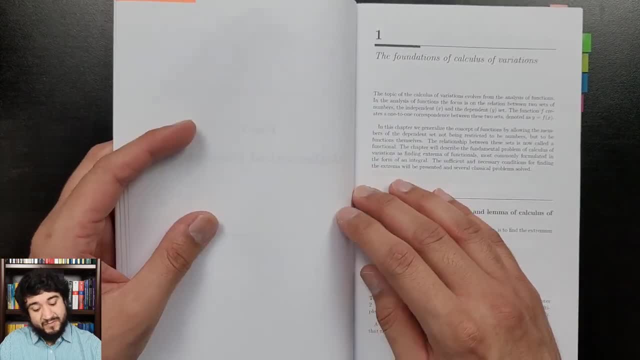 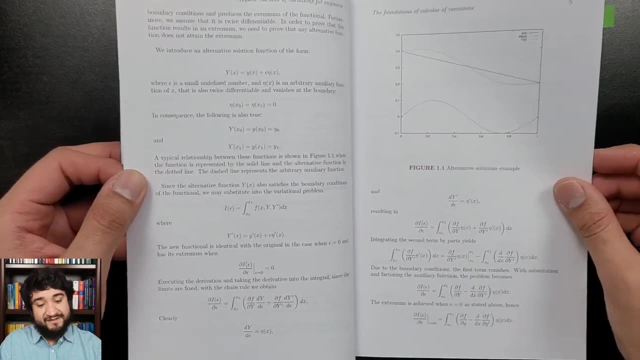 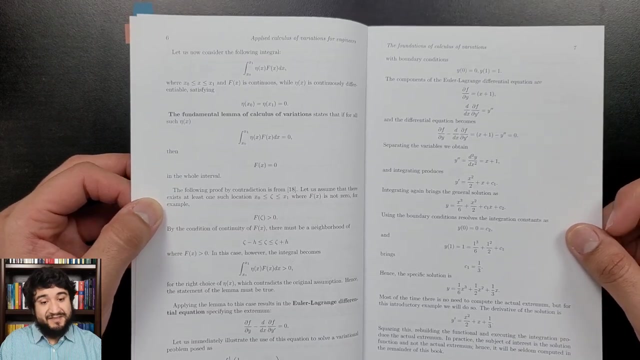 I think it can. the writing can feel lazy, So here we go: the first chapter In just a few pages. here the author derives the Euler-Lagrange differential equation And from what I've seen, that's nothing you're going to get in any other book, A lot of other books, what they tend to do. 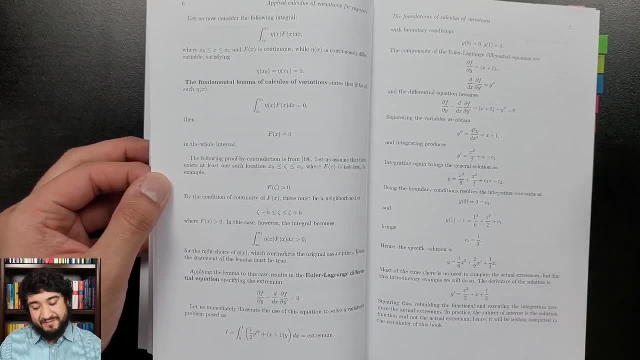 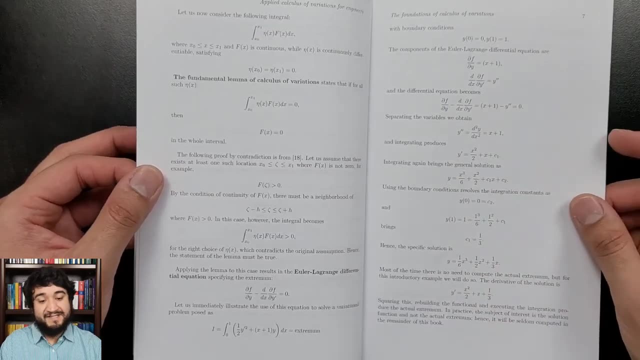 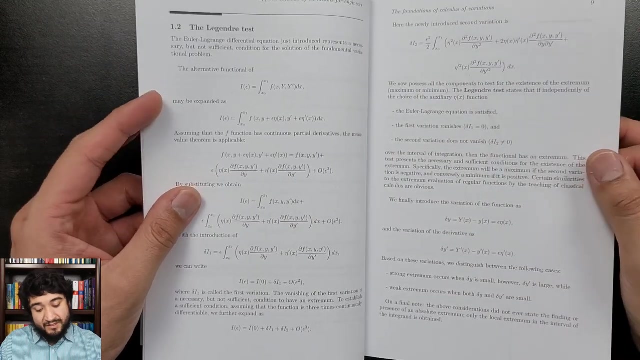 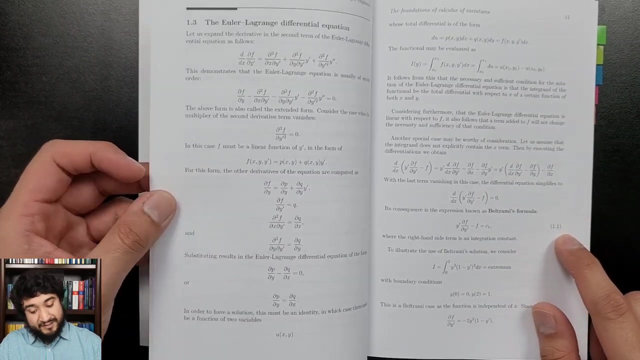 is go over a lot of mathematical detail. They want to talk about function spaces and all that Not here. Very quickly he gets into just the main concepts of calculus, of variations, One thing that irritated me very much when reading the book. look at this, here We're on. 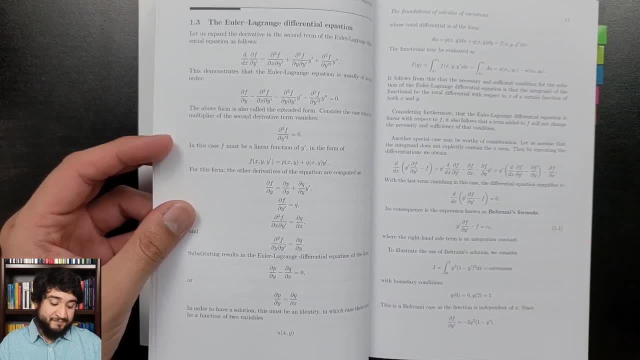 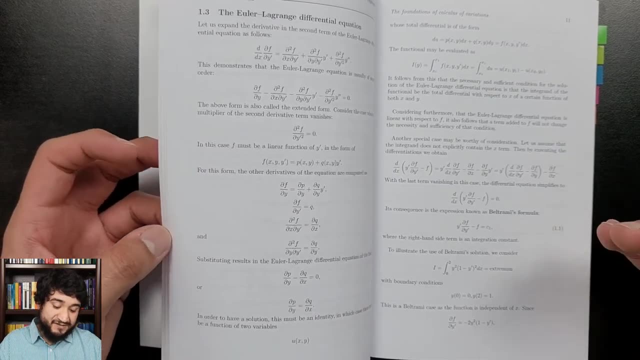 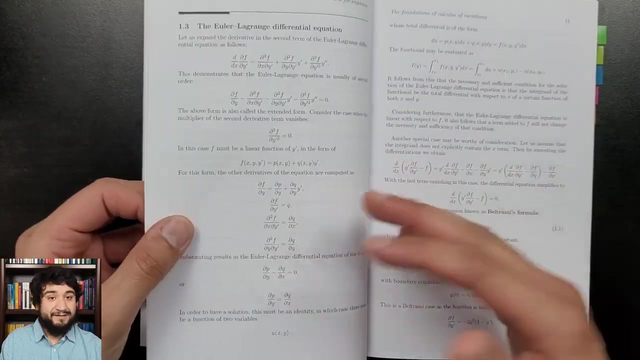 I don't know what page this is like eight, nine exactly, And this is the first numbered equation that we've got here on Beltrami's formula. He references the Euler-Lagrange differential equation and he did not bother to number it. Look, this is just something that irritated me when I was. 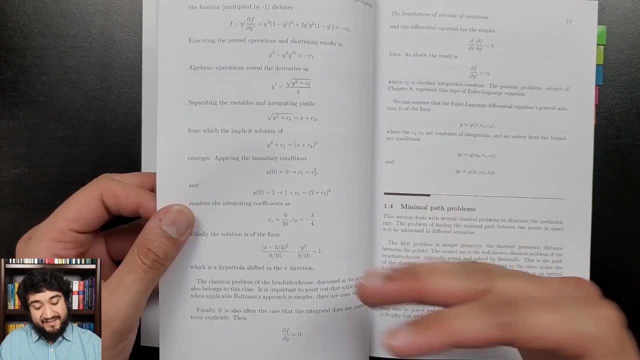 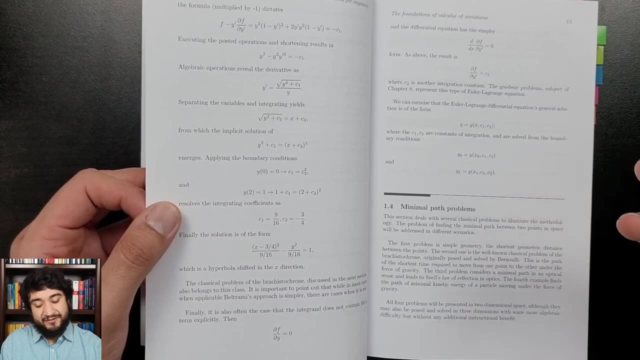 reading the book when I was taking notes. It's not that big of a deal, but that's one of the little things that make it feel lazy. Another thing that makes it feel lazy: lack of examples. I think there could be way more examples in the book. There are three in 30 pages. Now another. 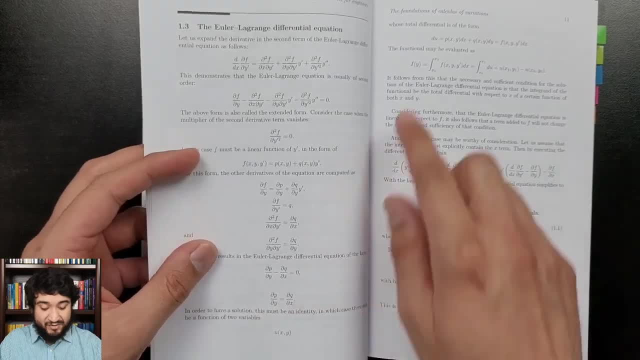 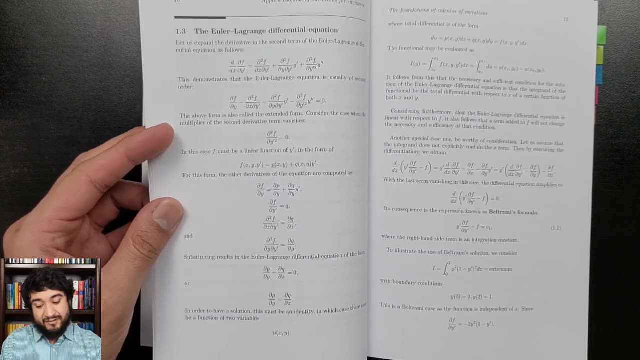 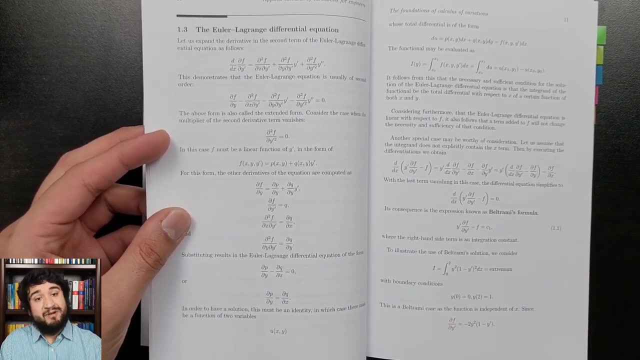 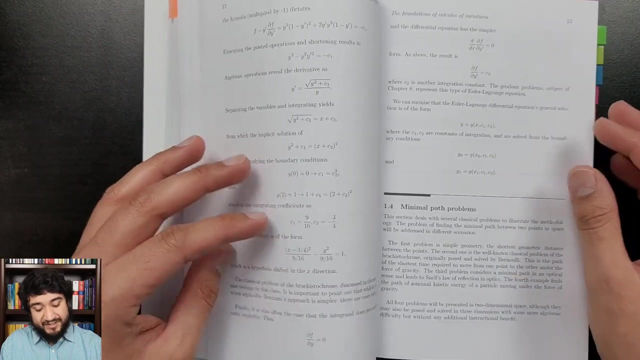 thing right here in particular. I wasn't a student that needed to use multivariable calculus for my work in university or afterwards, So maybe this is just something that I don't remember from when I took multivariable calculus, but this right here, this didn't really make sense to me, I'll be honest, but it really wasn't all. 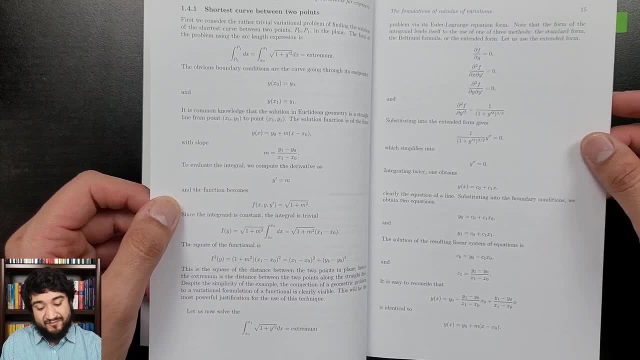 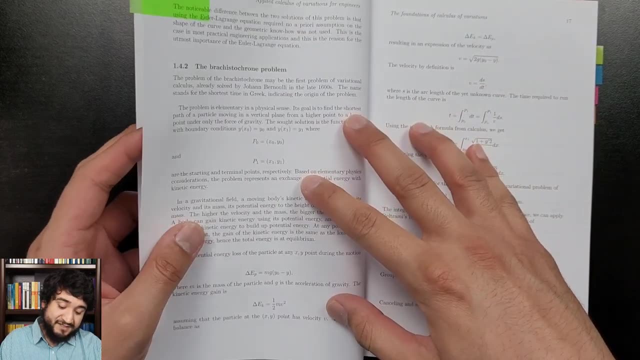 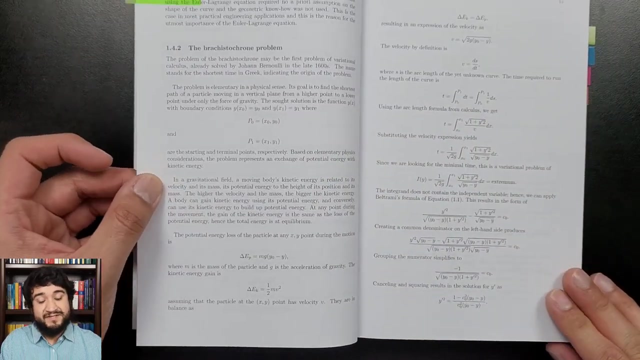 that important in terms of being able to solve problems or do some of the problems in this book. Now here on this section is where he gets into some applications. So this is the problem that basically started this entire field of calculus: variations, the Brachistochrone problem And I hope 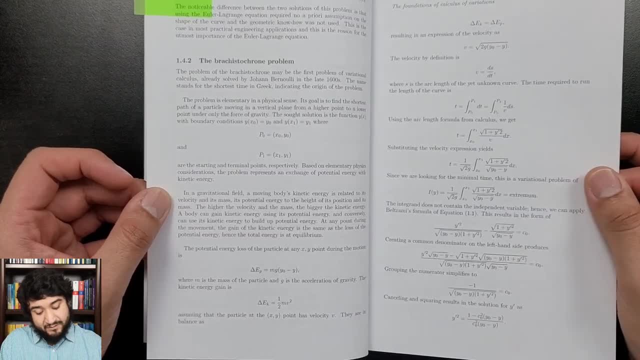 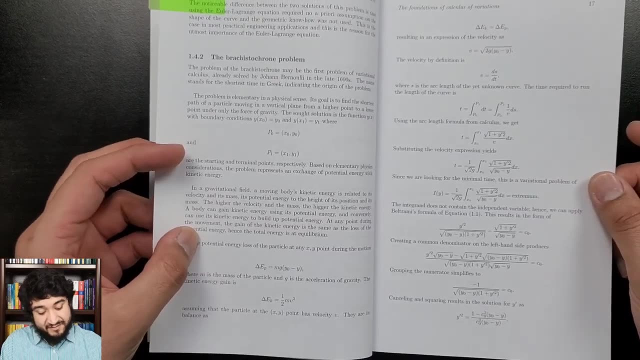 I'm pronouncing that correctly. So my physics background isn't very extensive, but I could follow this. I thought it was pretty straightforward. Again, if you don't, if you don't have any interest in physics, you just want the calculus of variations. 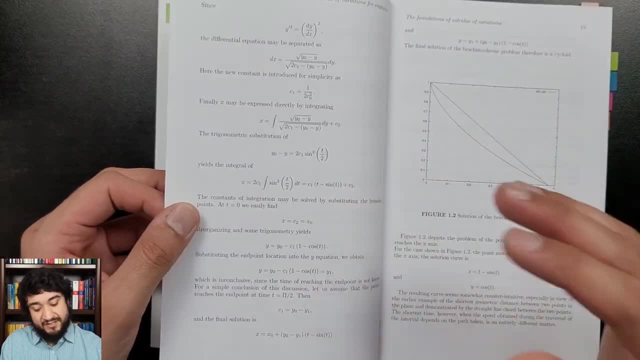 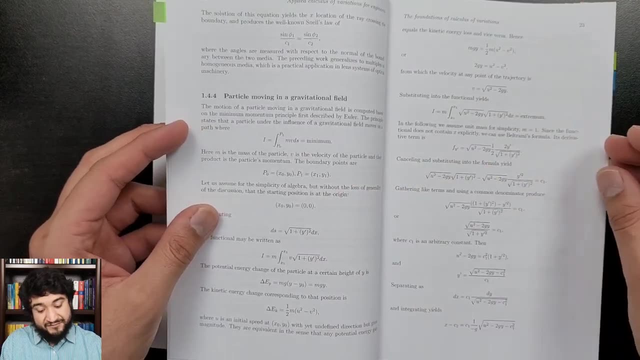 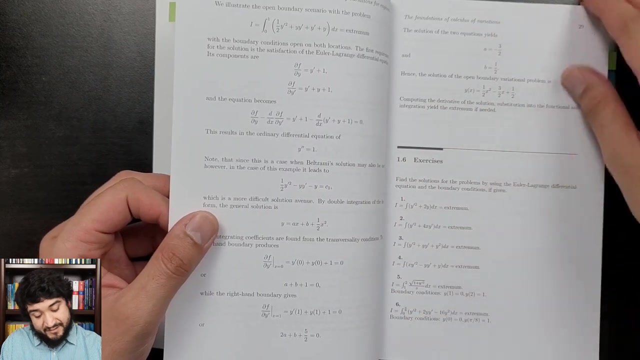 You can 100% ignore this section and the preceding two sections as well here on Fermat's Principle and Particle Moving in a Gravitational Field, And he's got one more section here at the end. And then they are the exercises which have solutions at the end of the book. 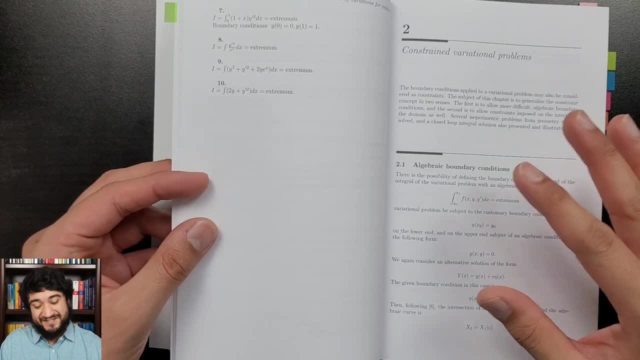 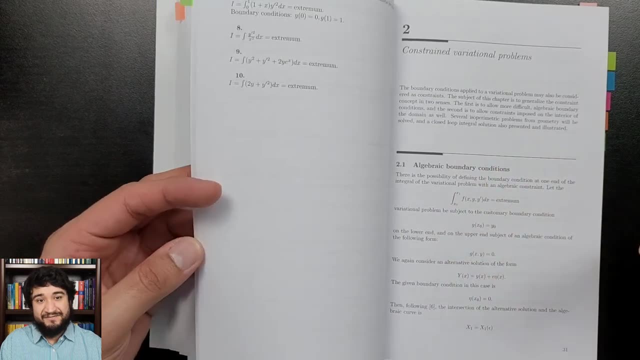 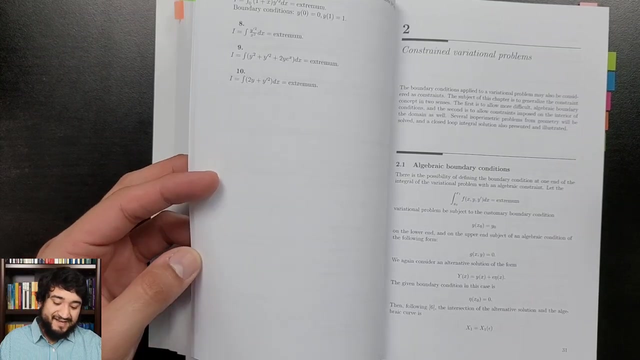 Here I need to give you all a disclaimer. Honestly, I lost interest in the subject after this first chapter. It's nothing towards the book. If you saw my last video when I talk about the DevNath book- the red one right there- you'll know that I did not like fractional. I don't like. 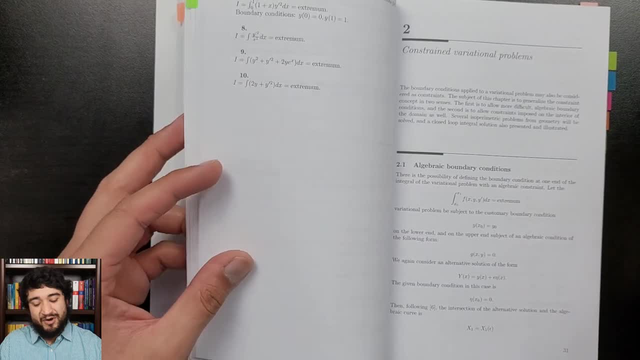 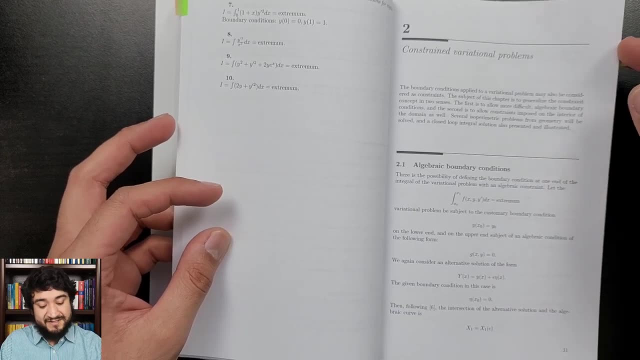 fractional, partial differential equations, Like it's just. they're just types of problems that I personally don't like working on. So I have not read the rest of this, but I skimmed through it to find some important sections, or some sections that I think are important to me. So I'm going to 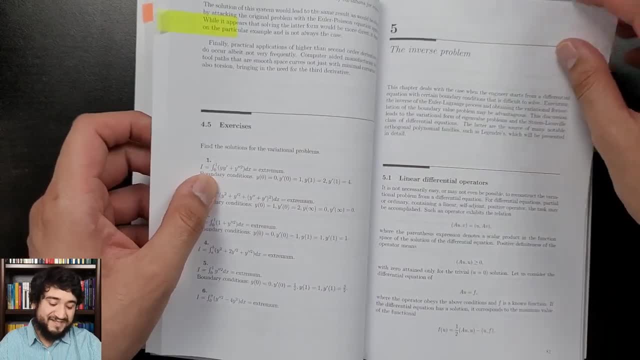 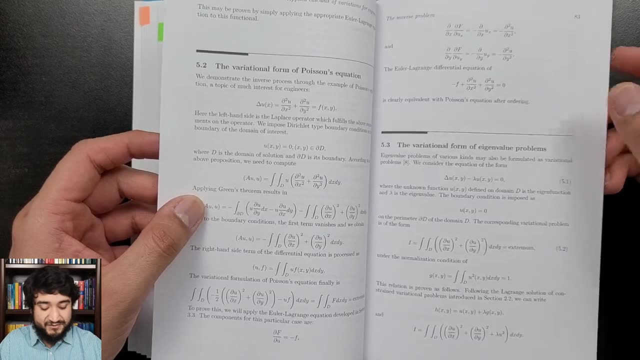 go through them one by one And I think engineers will find important. So that's the end of my disclaimer there. So here chapter five, the inverse problem, And I think the engineers would find this useful as applications to partial differential equations. Same this chapter here. 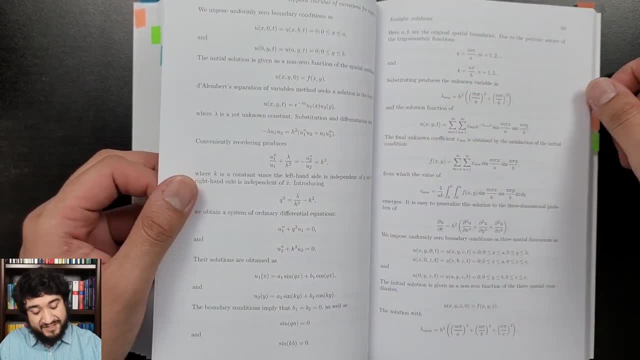 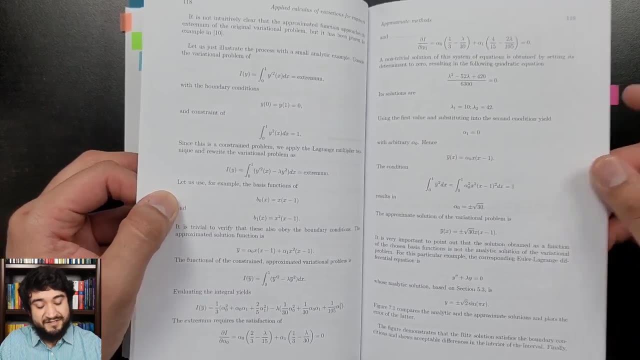 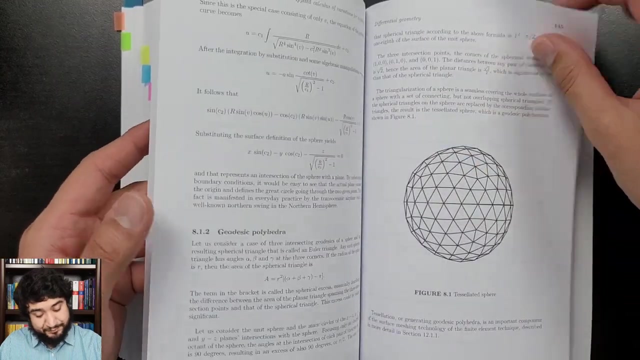 on analytic solutions, also some partial differential equations, applications, And there is a section here on approximation and numerical methods that I think you will also find interesting. Second half of the book on modeling applications. Here he gets into some differential geometry. The next chapter he goes over computational geometry. 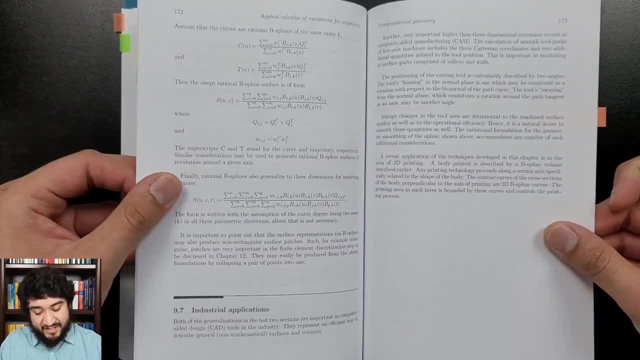 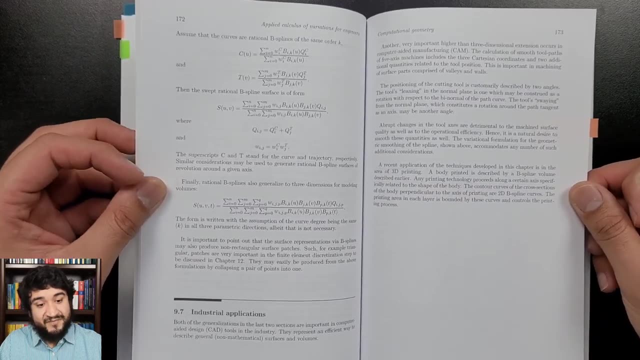 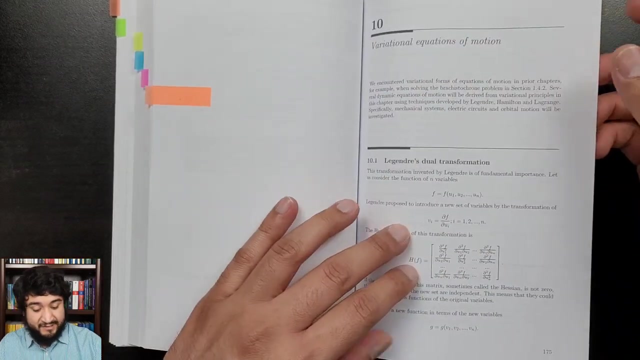 I think the end here of this chapter has this section here on industrial applications that I think you all would find motivating in terms of trying to read this book or being interested in reading this book. And here he gets into some. I don't know if it's technical, but I never got to. 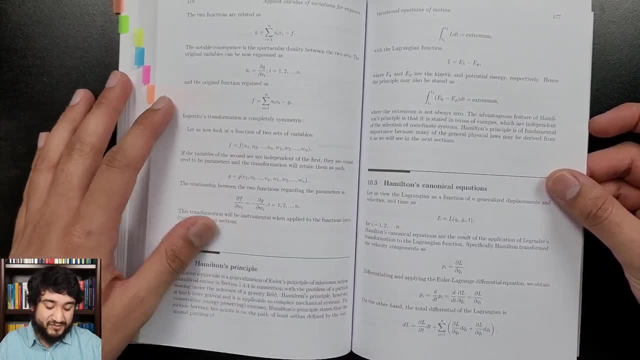 classical mechanics, which is a little bit more complicated than I thought it would be. So I'm going to go over some of the technical mechanics. which is well. I guess it's extended to quantum as well, but I never really talked about or learned about Hamilton's equations, things like that. 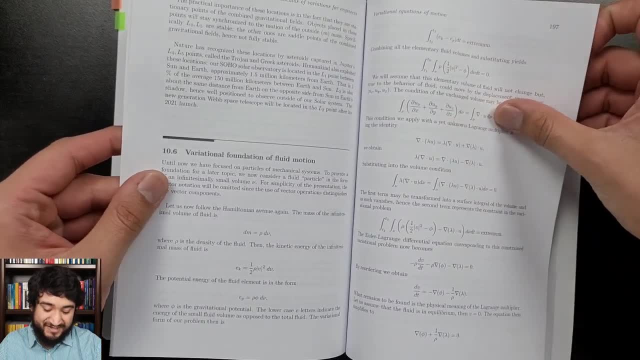 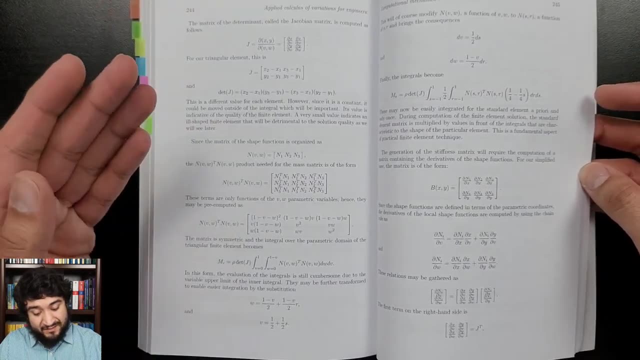 I saw some orbital motion stuff which seemed pretty interesting: Fluid motion, analytic mechanics. here Again, if you want to understand everything in this book, you're going to need those four or five things that I said in the beginning For the first chapter. 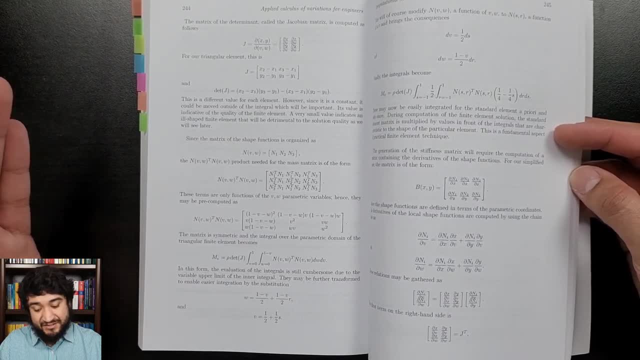 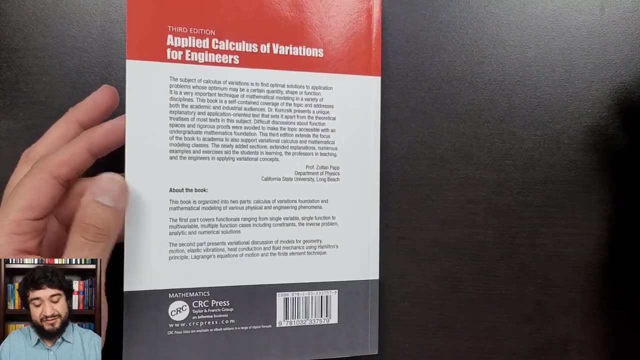 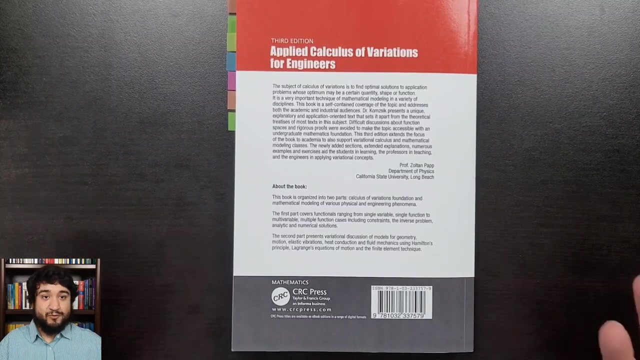 you pretty much just need multivariable calculus. As the book goes on, you will need more linear algebra, ordinary differential equations and then partial differential equations, and that should be sufficient. But if you want to take advantage of all of those physics applications, of course you're going to need some physics, I believe he 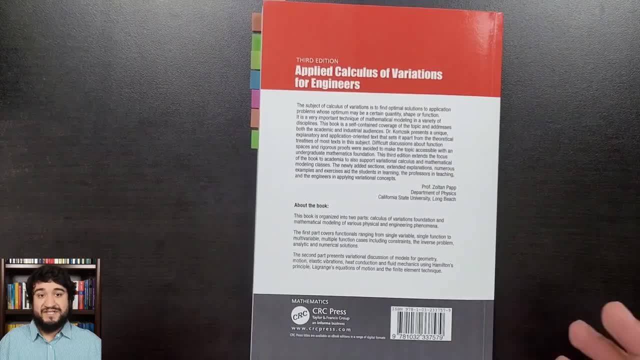 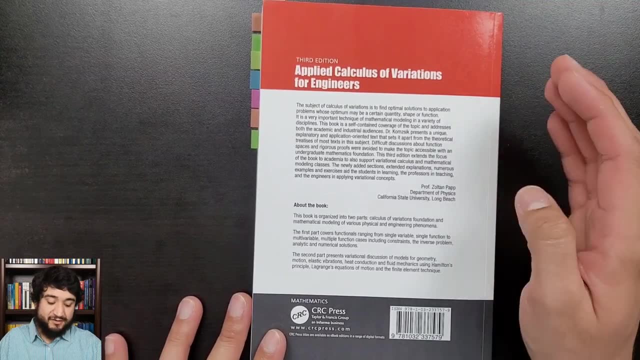 says here in the back of the book and in the preface that the book was originally intended for those in industry, so the professional, the practicing engineer. So it's kind of assumed that you already know all of that. But yeah, hopefully you all find this book. 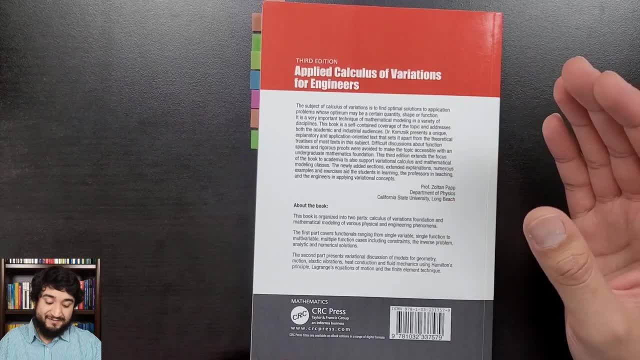 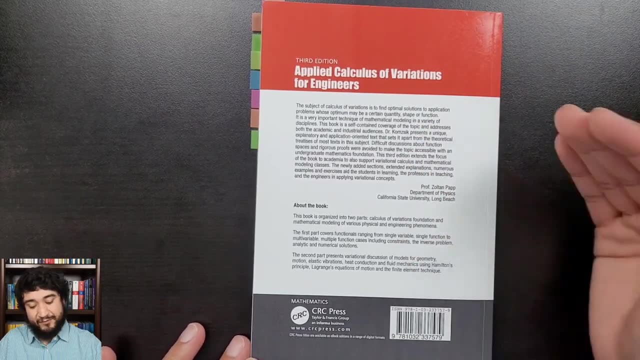 interesting. I thought it was awesome. the first chapter. I thought it was unique. I've seen nothing like that first chapter in any other book. They kind of just want to force feed you function spaces in every single book on calculus variations I've seen. 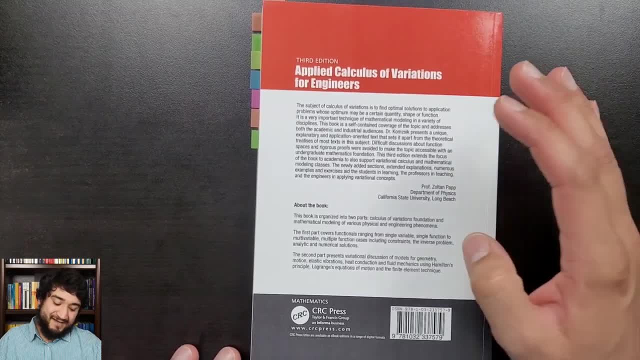 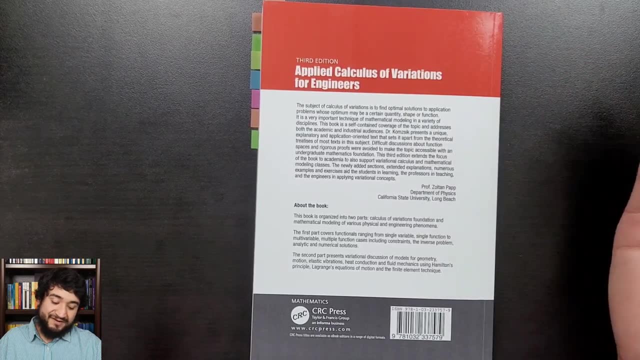 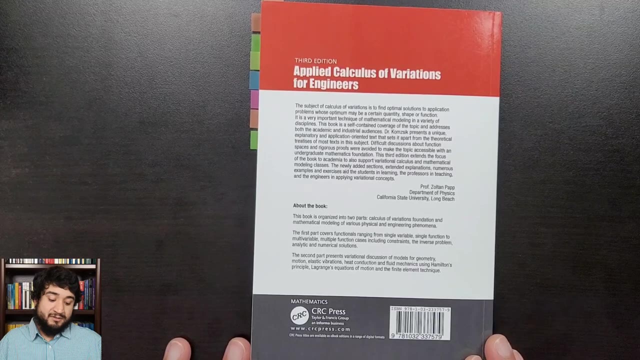 Maybe not every single, but a lot of them do. So, yeah, I like this one a lot. I hope you all find it useful as well. You all that are engineers. let me know if you think this is useful to you or will be useful to you. I've got a couple of more videos, or a few more videos. 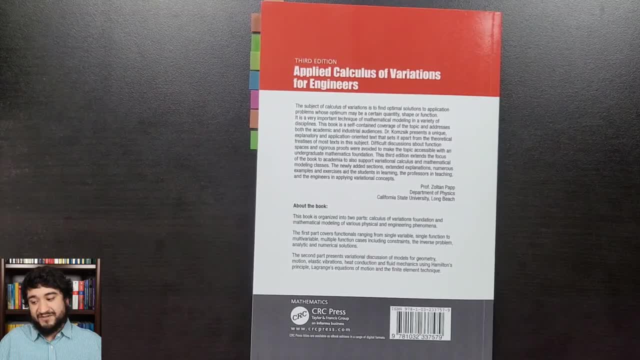 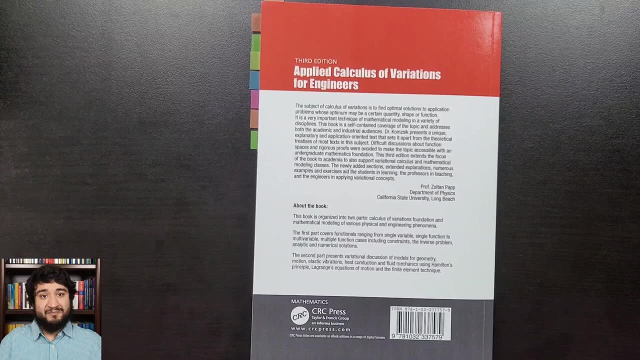 that subscribers have requested topics on or me to do books for. So yeah, I've got foyer series coming up, complex analysis. after that I've got a book on discrete math as well coming up. And then another subscriber asked me for some Adomian decomposition, nonlinear differential equations. So yeah, if you've got requests.